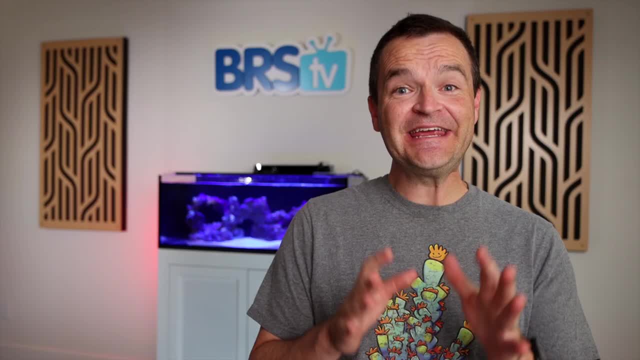 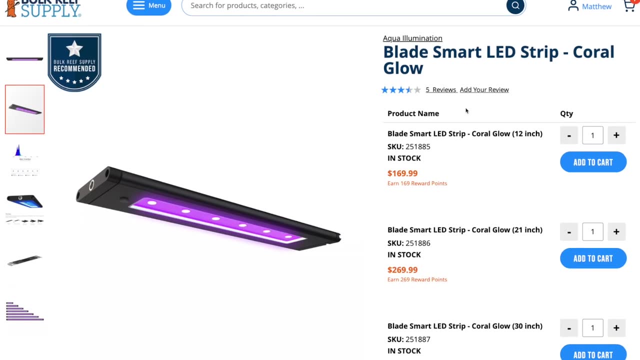 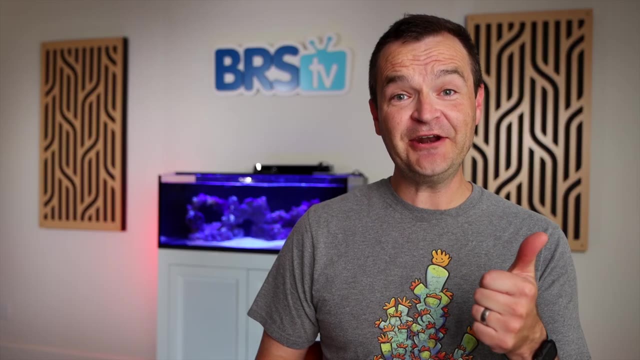 behind lighting. we'll save that for the next beginner series. here are the lights we chose and why we chose them: Three aqua illumination blades, two grow and one glow. Why not just one blade, which honestly would have been enough for this tank? Two reasons: shadowing and spread. 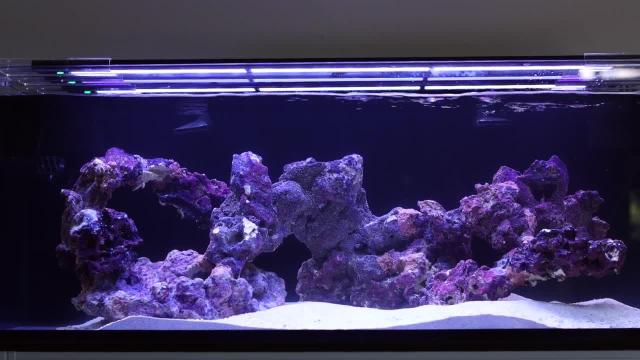 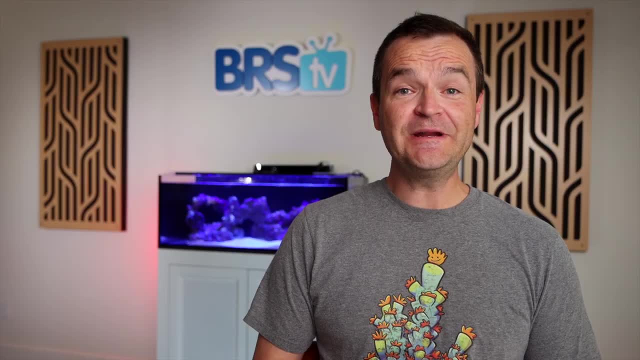 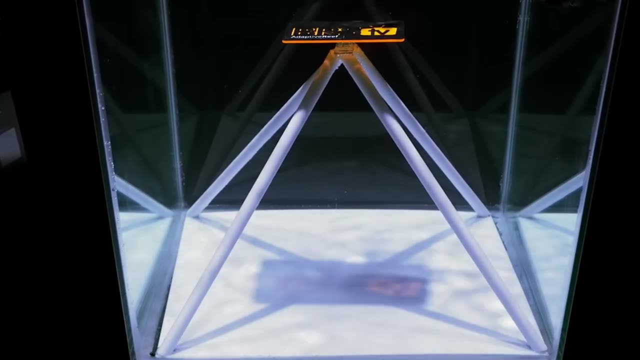 We want an even blanket of light throughout the entire tank and we want the option to grow coral anywhere in that tank. so three lights means complete coverage. Three lights also means shadowing will be at a bare minimum. The BRS Investigates team did some pretty eye-popping. 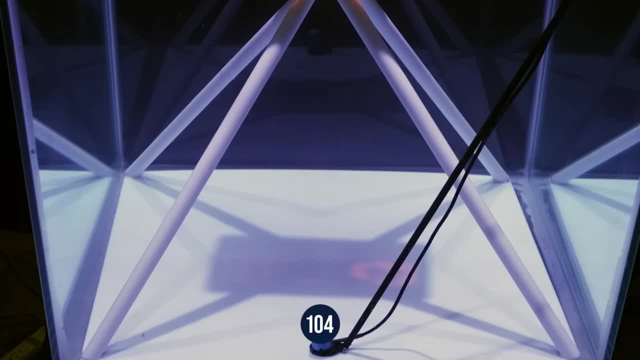 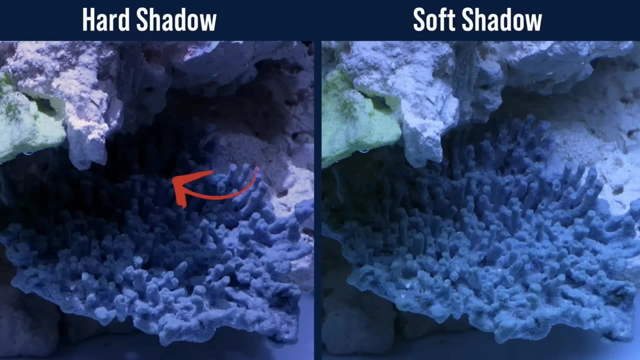 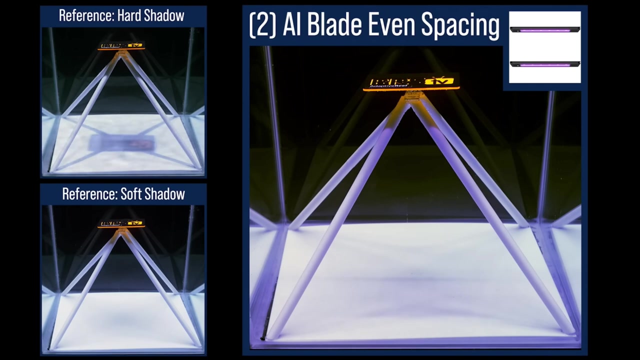 experiments on a whole host of different lighting configurations and the different shadows they created. Large shadows create areas in our tanks with significantly less light, which can be detrimental to coral health and coral growth. Using multiple strip LEDs like the AI blades significantly reduce shadowing. We also like the blades because they're just really easy. 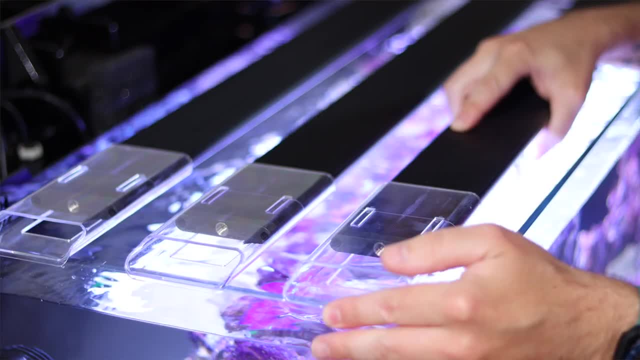 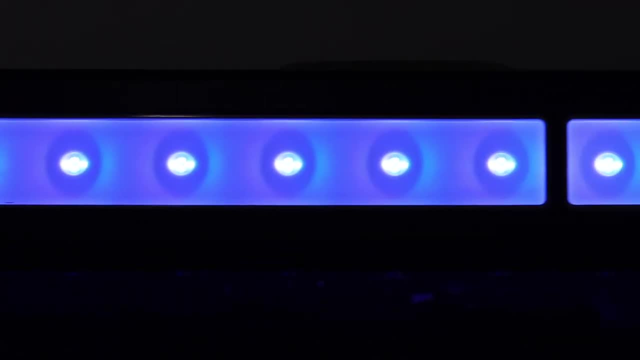 to mount The included tank rests means we can place the lights directly over the aquarium. We chose two grow blades because they are designed to grow coral and one that is basically good for glow blade, because that glow will help make coral fluorescence absolutely pop. 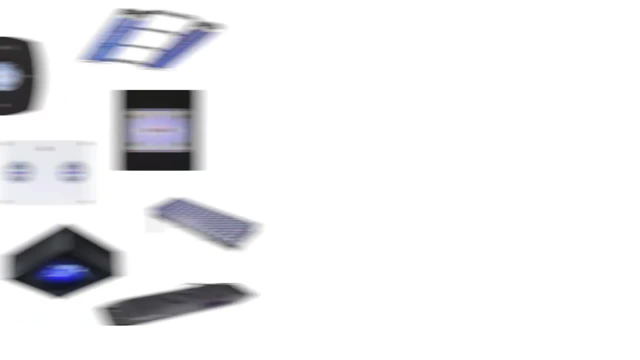 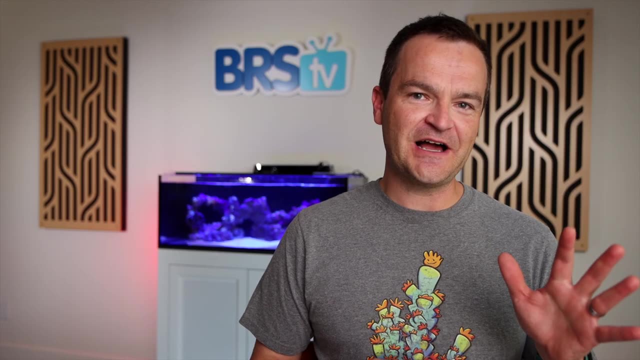 Before we set up these lights, a couple of quick points. First, there's probably around 25 different lights that would have worked well over this tank. There's a light out there to fit every design and every budget. so if the AI blades 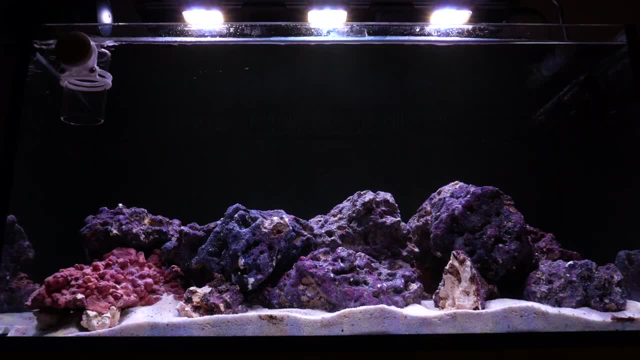 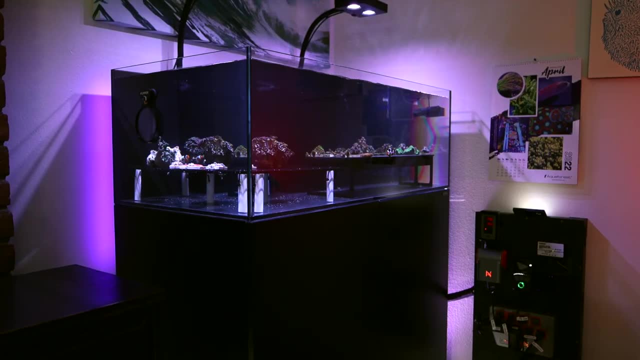 aren't for you, don't fret, There's definitely good options out there. And secondly, the hardest part is just choosing the right light. If you feel lost, just find a tank that you like and copy it. We've set up many successful. 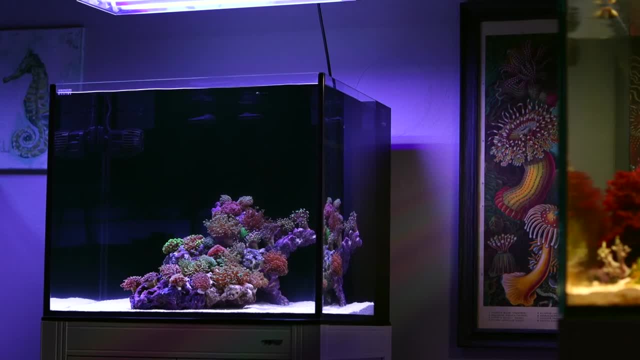 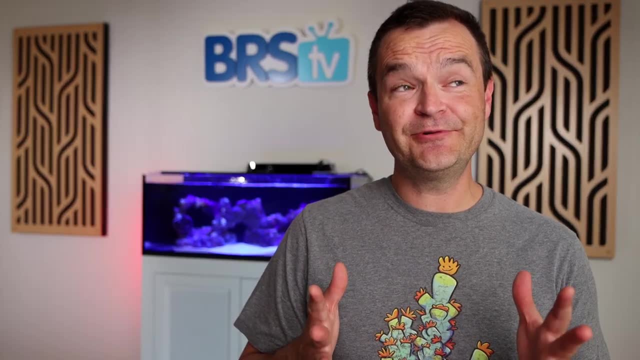 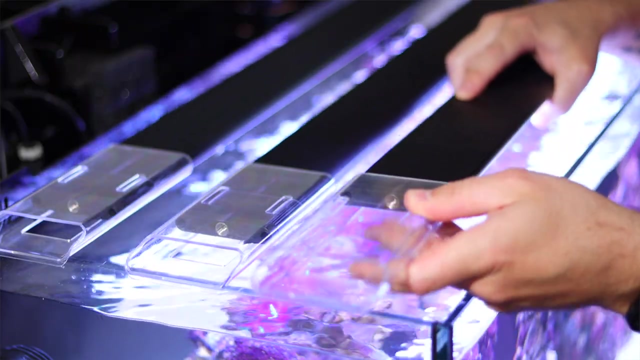 tanks here at BRS. so if you need some inspiration, just scroll through our playlist, find something you like and copy the lighting setup. Setting up these lights is really ridiculously easy. These are the 30-inch blades, and setup literally just means sliding the tank rests into place and resting them on top. 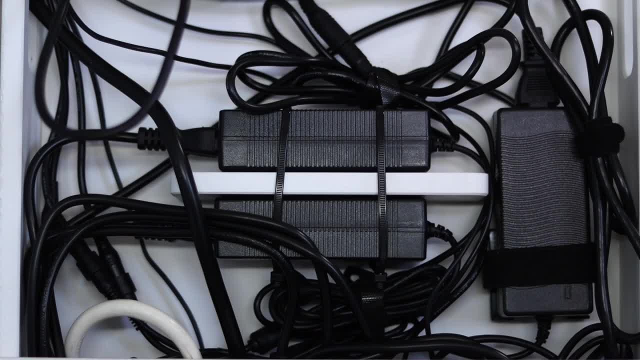 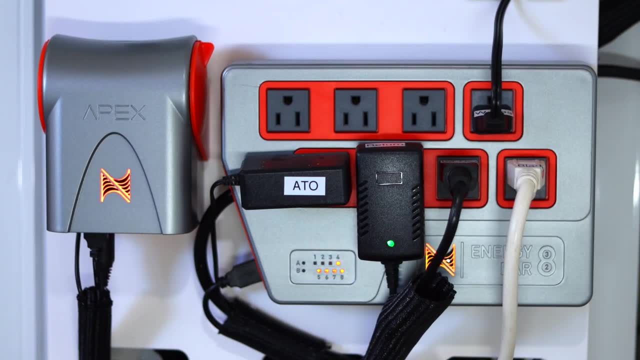 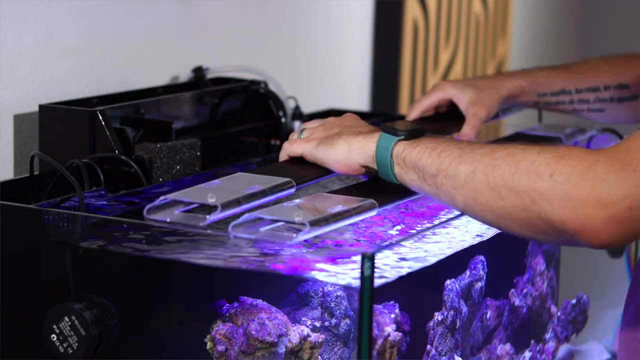 of the glass. I used Ecotech power supply brackets and the Adaptive Reef control board to clearly organize the wires and used a small extension cord to tie all three of the lights together so I could plug them in to a single outlet. I placed the glow in the middle and the two grows in the front and rear of the aquarium. 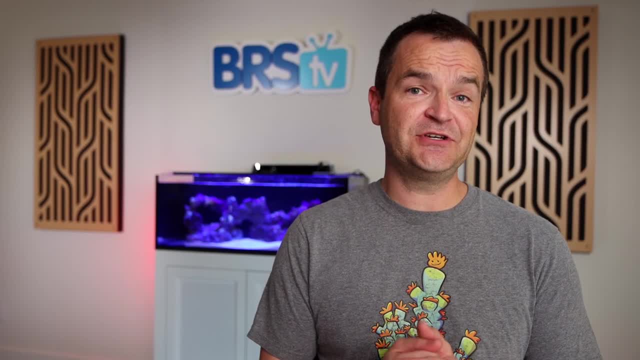 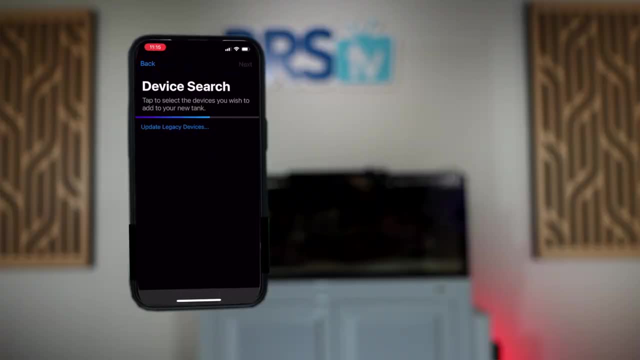 You can either use the My AI or the Mobius app to control the lights, but I went with the Mobius app because I have some other Ecotech products already set up within it. Add the light to your new aquarium and now it's time to program. 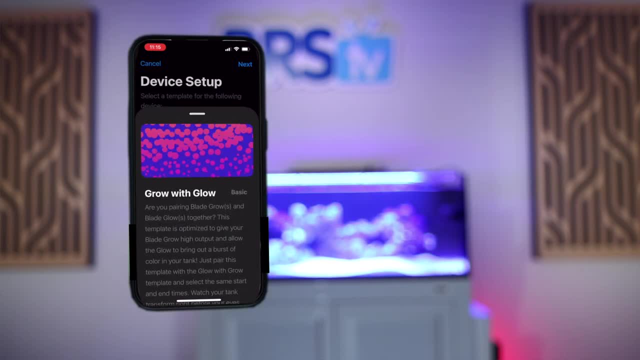 Luckily for us, the Mobius app is software-enabled. It's available in. the Mobius app has specific templates for this exact setup. It's called Grow with Glow. To set this up first click on the Grow lights. select Templates. click on Grow with Glow. 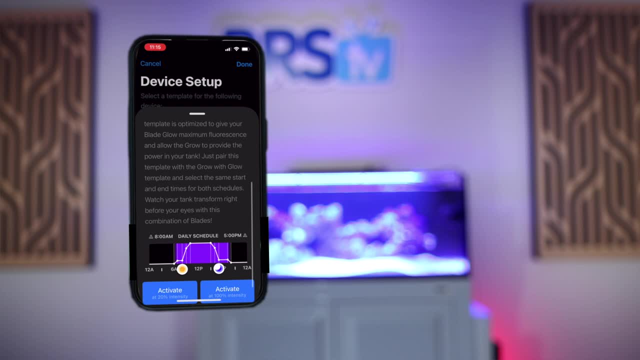 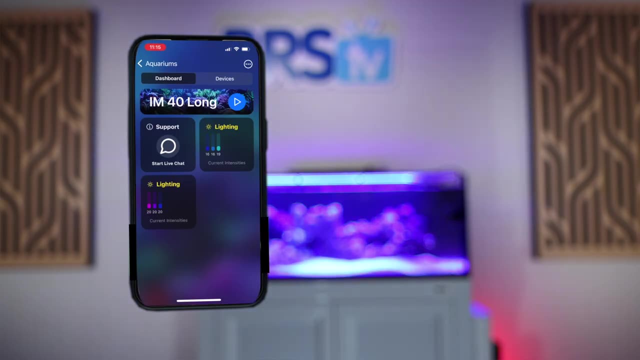 and activate at 20% intensity. Then return back to the aquarium screen. click on the Glow light Templates- Glow with Grow and activate at 20% intensity. The preset schedule has a slow ramp from 6 to 8 am. then ramps up to full power for five hours, from 10 am to 3 pm, a quick ramp down until 5 pm, followed by a sunset cycle until lights off at 8 pm. I usually end up playing around with the lighting schedule. 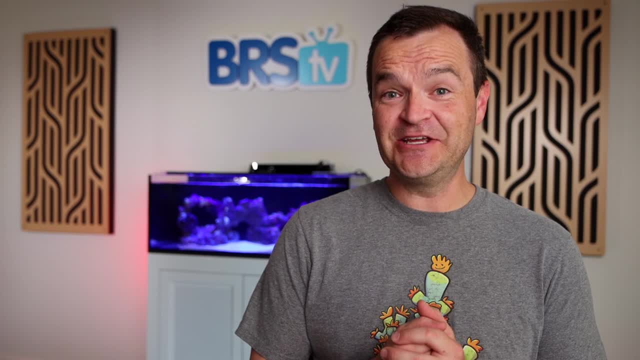 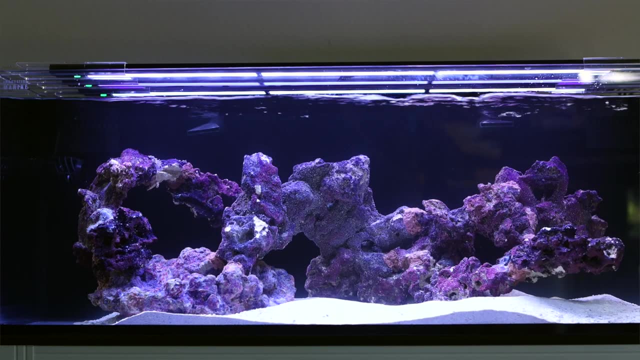 but not this time. I trust the AI and ecotech lighting gurus to create a good schedule, so I'm just not gonna mess with it, But I do need to make adjustments to the lighting intensity. Too much light will not only cause nuisance, algae growth. 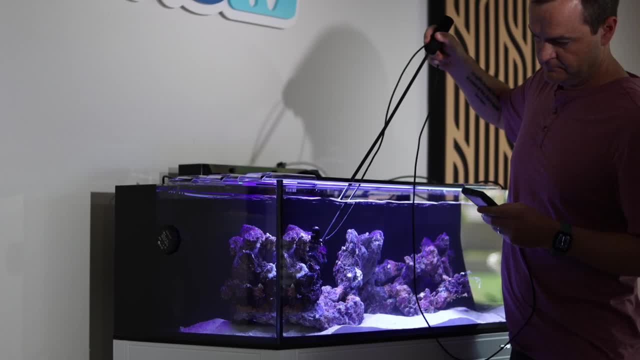 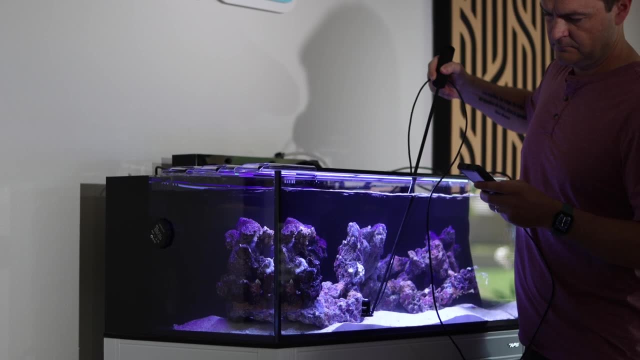 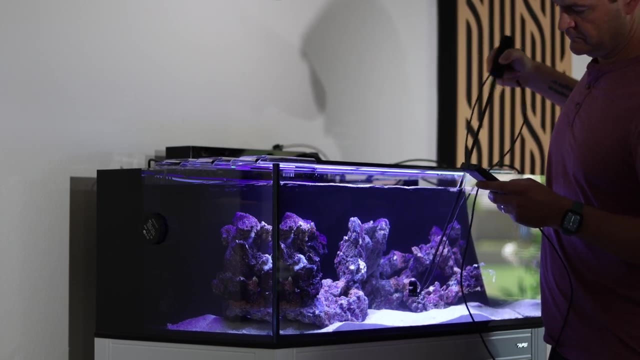 but it can also kill our coral. Using a PAR meter, I turned off the return pump and wave makers and took readings all throughout the tank At the 20% preset intensity. I chose PAR readings ranged between 20 and 60, a great range for fish and soft coral. 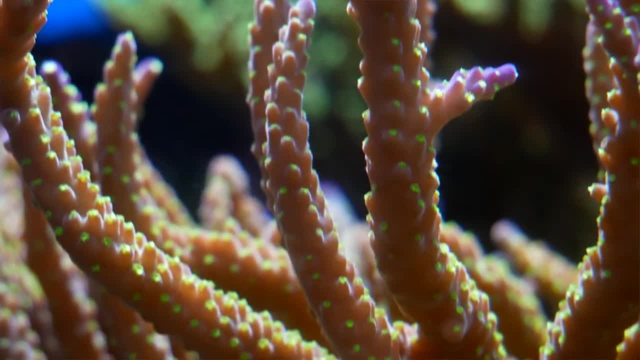 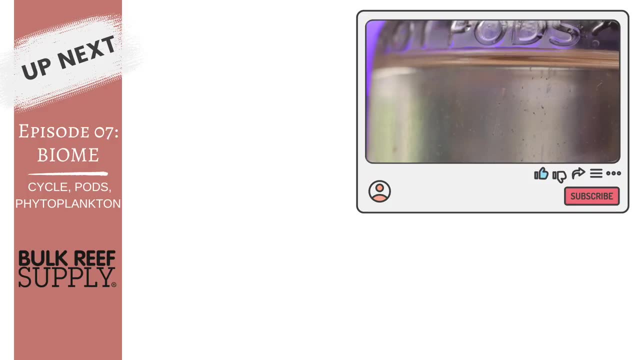 If we decide to add some stony coral in the future, we will have to increase the intensity. Now that the lights are on, we can be sure of one thing: the uglies are coming. But what if there was a way to minimize? 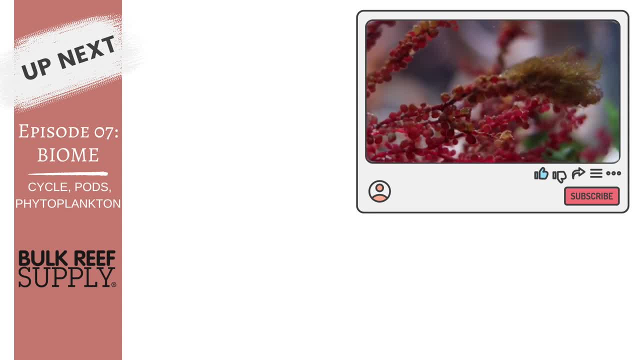 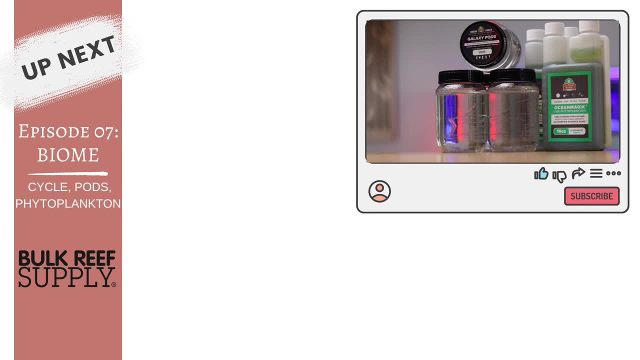 or even completely eliminate the ugly diatom from ever occurring in our tanks. Would you be interested? Well, there is, and we'll show you how to do that right now in episode seven. Thanks for watching. happy reefing, be well. and we'll see you next time. 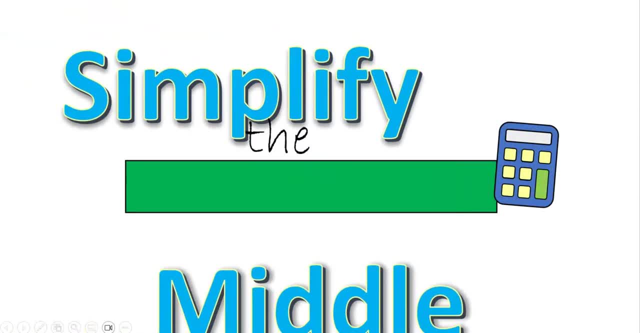 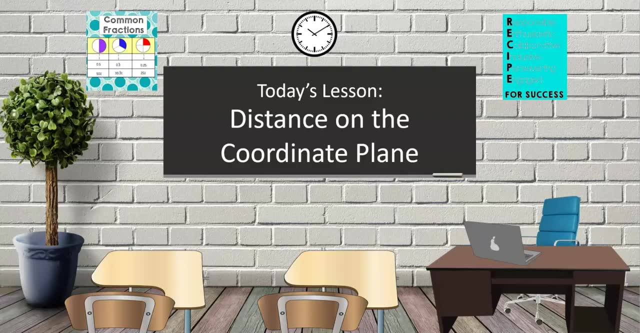 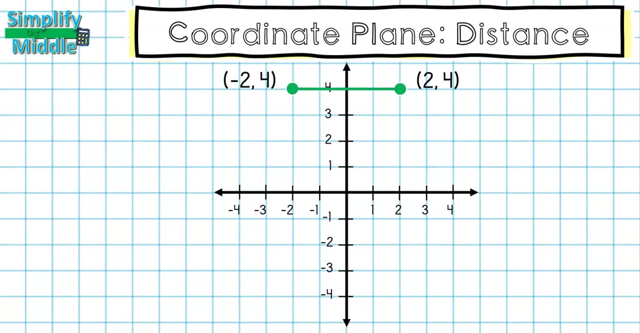 Hi and welcome to today's lesson: distance on the coordinate plane. Here we have a couple of points. Today we will learn how to find the distance between points like these, but first we need to identify if a line is horizontal or vertical. This line is an example of a horizontal line.